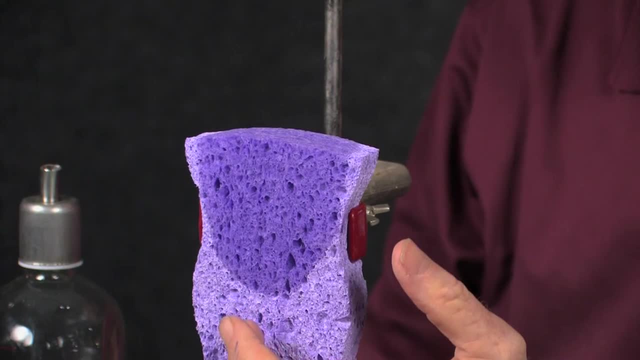 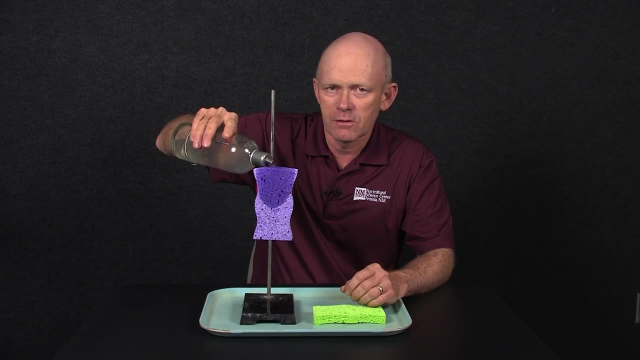 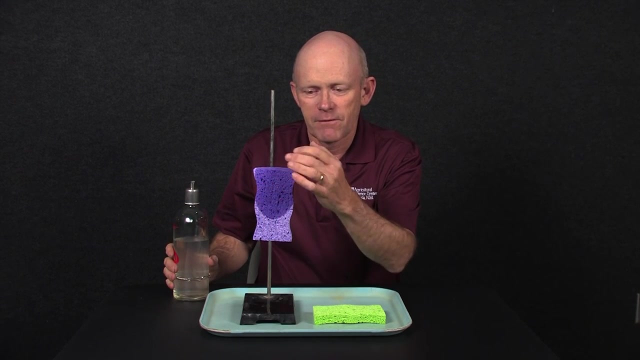 water infiltrates into the soil. it's going to infiltrate down through the soil profile And now, as we keep adding that water, another term that to introduce is called percolation. So our water is percolating through our soil. It's filling up the large pores that are in the soil and then, as those pores, 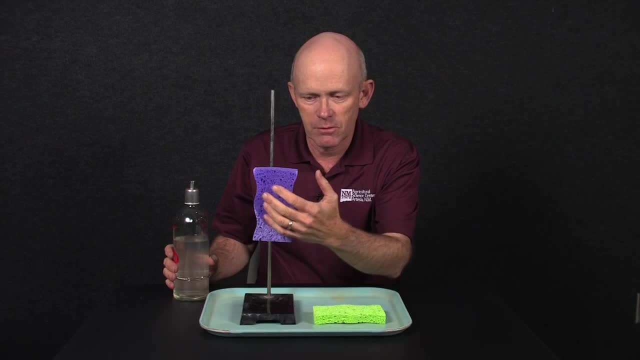 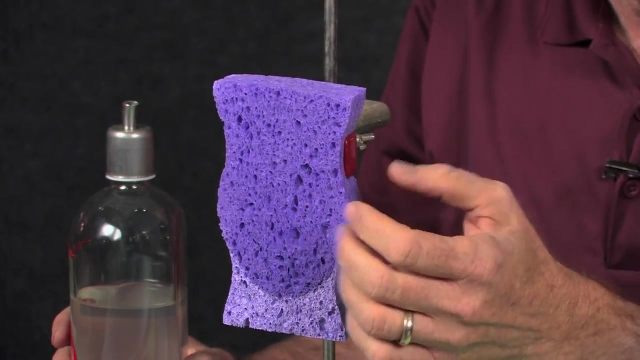 drain air fills up those pores. So that's going to be that percentage of the soil volume that is our air spaces. And then there's some smaller pores and then they can drain. over time They take a little longer for them to release that water. 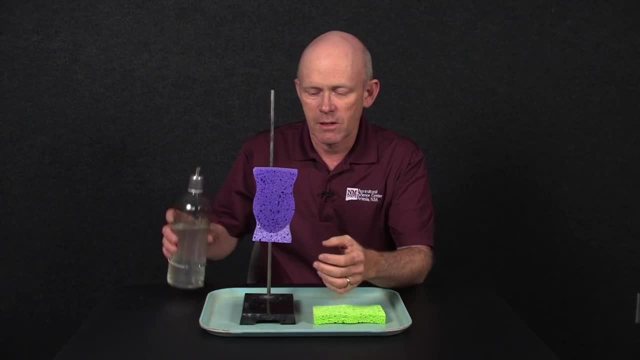 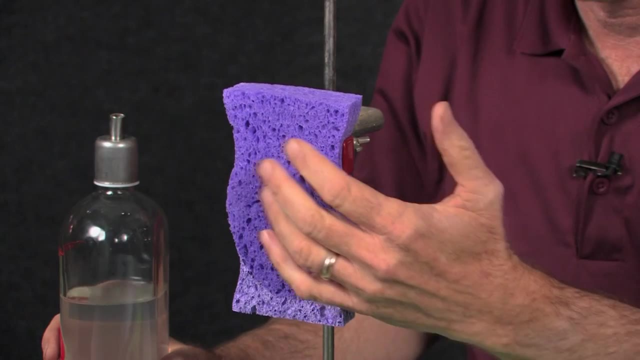 that water to move through, and then it fills with air as well, And often we don't put enough water on. Some of our folks will irrigate their soil, but they don't put on enough water on and they leave a dry zone down here. 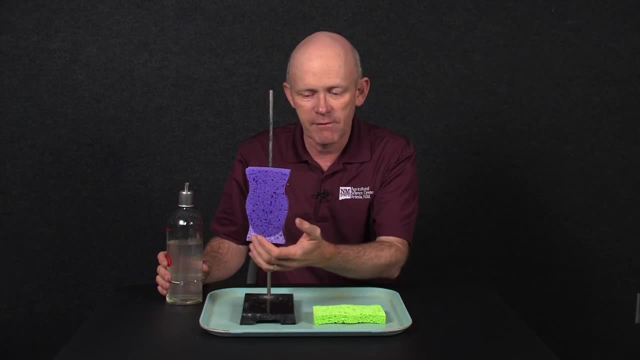 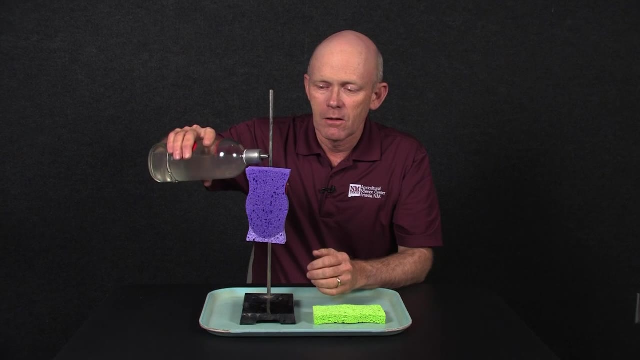 And if our plants are larger, they're not going to have access to the full volume of soil water. It's actually limited by how much water was put on, So we want to be able to add enough water to fill up that profile where we expect our plants. 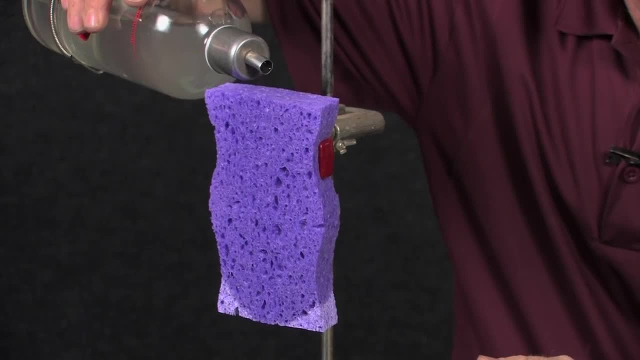 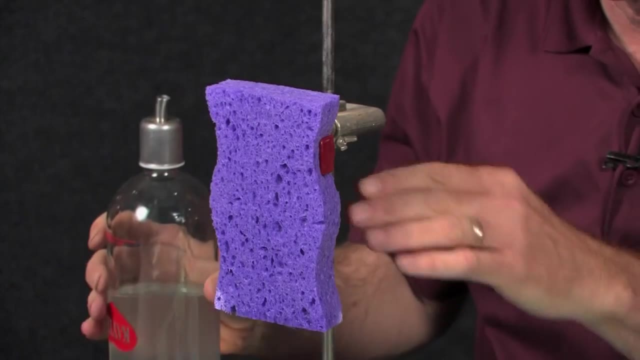 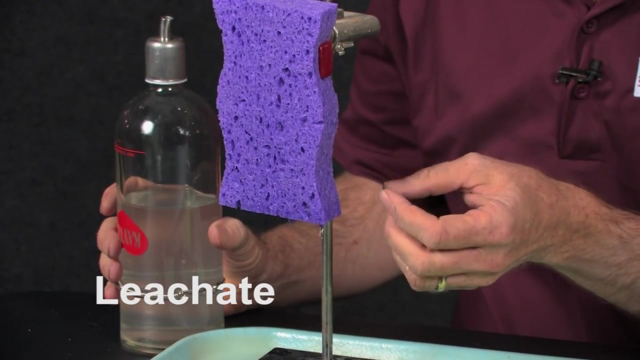 to get water from. As it comes, along with more water being added, it's going to start to reach the bottom of this top part of our soil. This water now can be referred to as leachate or drainage water, and it's going down into that second zone of soil. 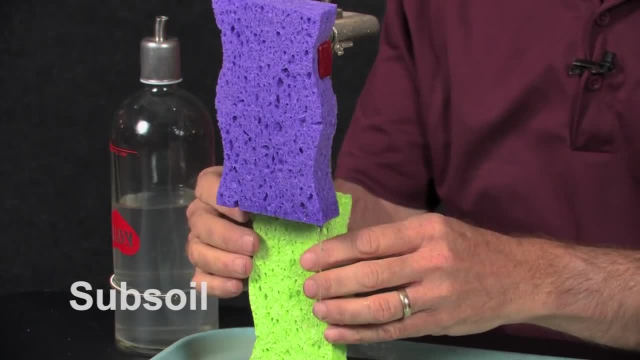 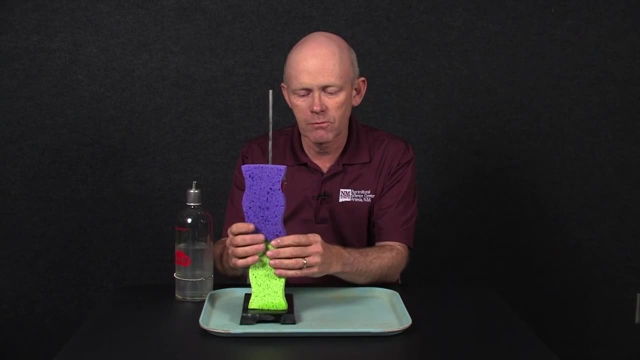 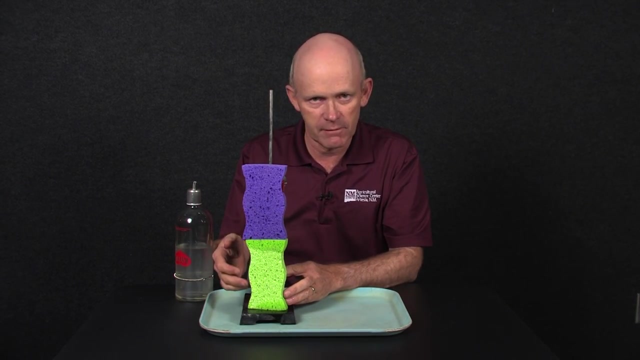 So this sponge is going to represent my subsoil and this is where we a lot of times when our irrigation water needs to be managed. we want to be able to move that water down into this zone of the soil, which is the subsoil, or the second foot of soil. Many roots will grow. 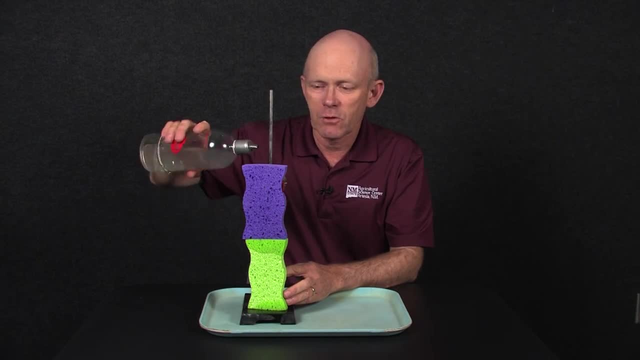 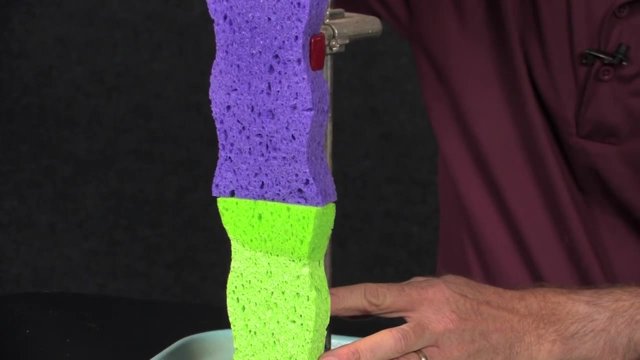 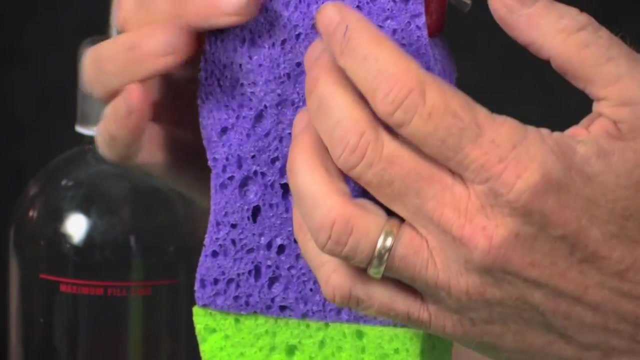 down to this depth later in the season and if we ever are short of water in the topsoil, we want to certainly have enough water in that second foot in order for the roots to take that up. So as this percolates through, we're now getting that water to drain down into. 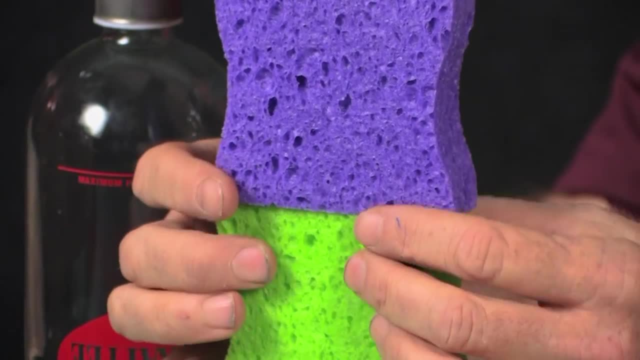 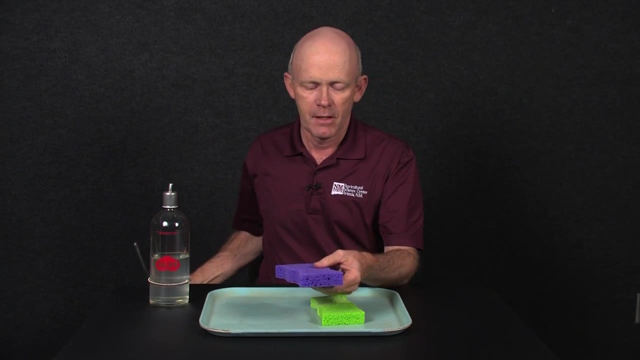 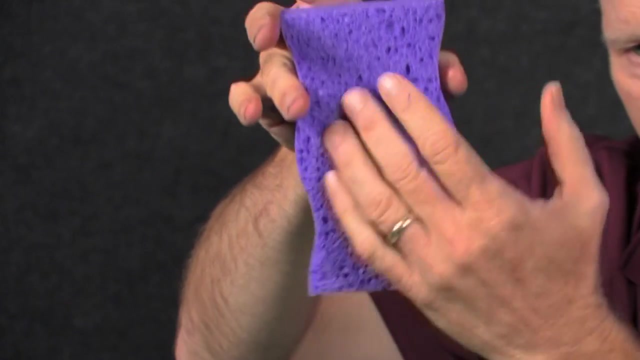 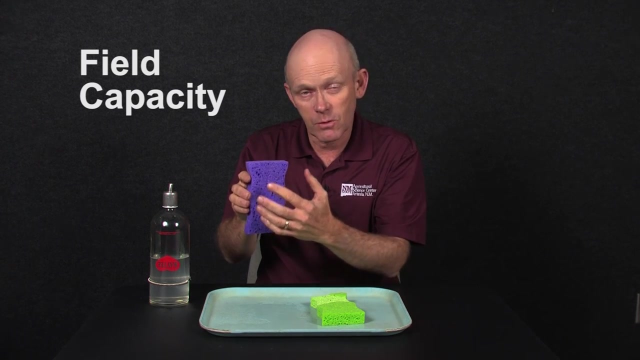 the second foot and this zone will start to fill up with more water. I want to switch to just looking at our top surface soil and that top surface now is pretty much drained and this is as much water as this soil can hold, and we call that field capacity. That's the amount of water that the soil will hold after all. 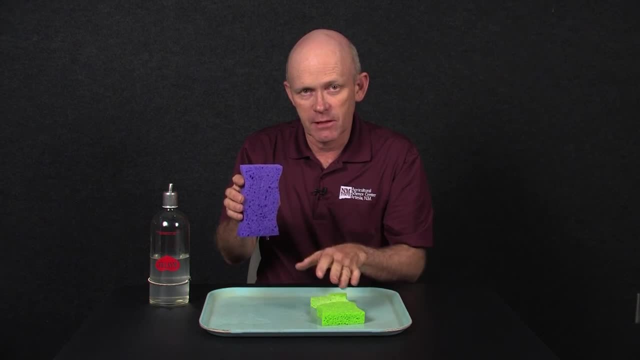 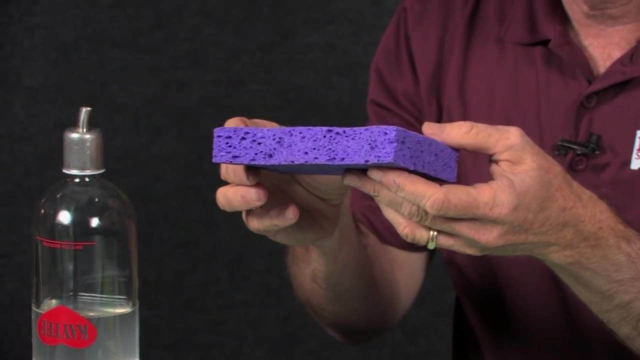 these pores have opened up and drained that water down to the soil, The second foot. So at this point it's field capacity, It's the most water that a soil can hold, Clays hold the most total amount of water and sands hold the least. 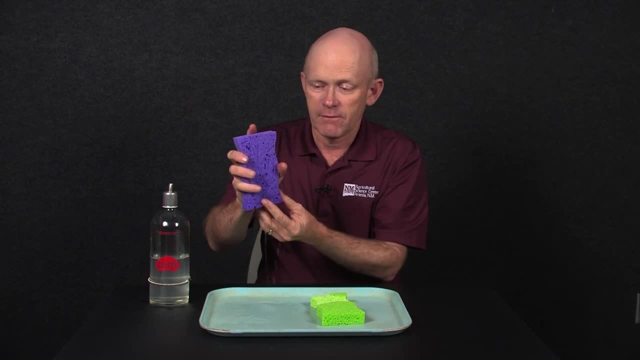 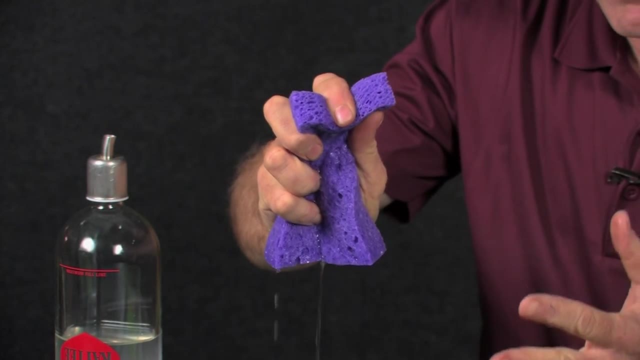 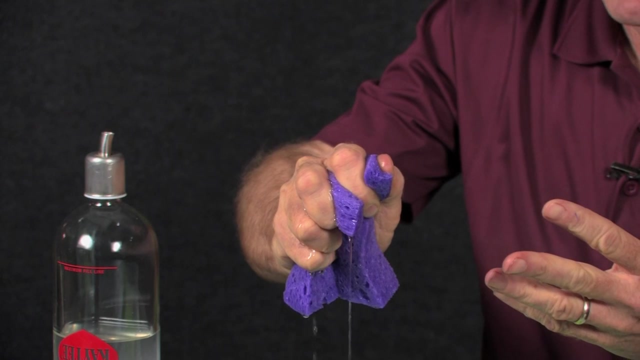 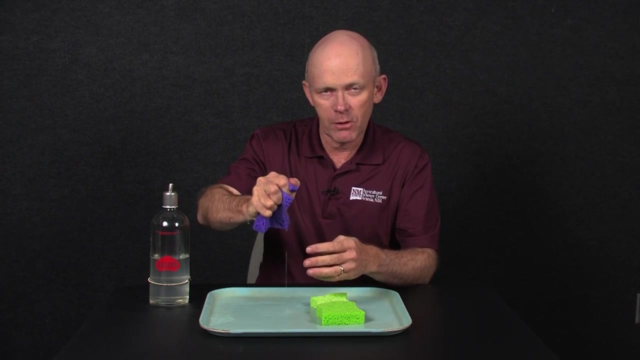 Then plants have then the ability to start extracting that water, and as it extracts that water, it doesn't take much effort to for that plant to remove the water. There's many plants that are capable of taking water out of the soil as it gets drier and drier, So at some point though, 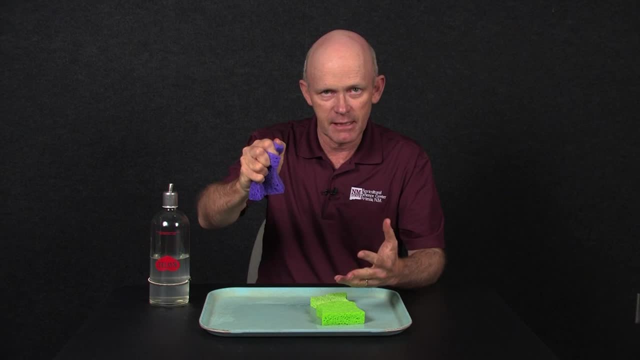 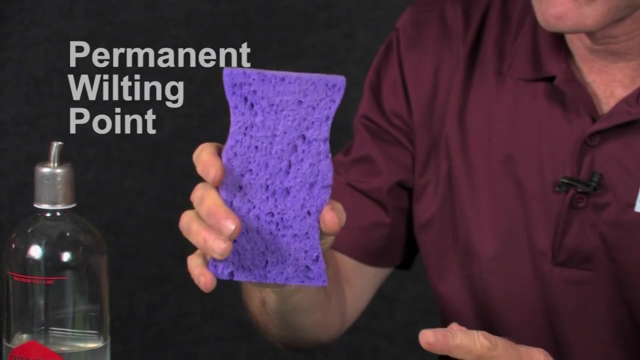 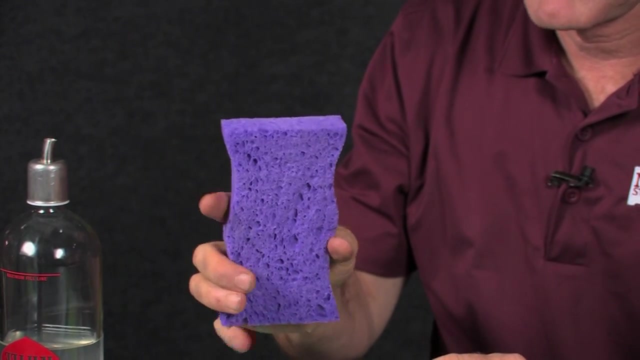 some plants just cease to actually be able to take any more water out, and this point at which plants cease to take water out of the soil is known as the permanent wilting point. Now, that number or that amount of water that's left in the soil is different for different plants, because there are other plants. 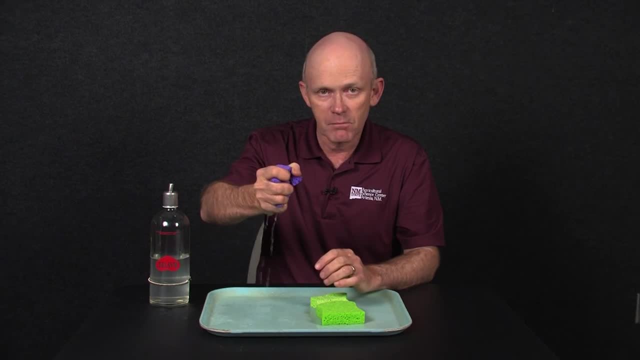 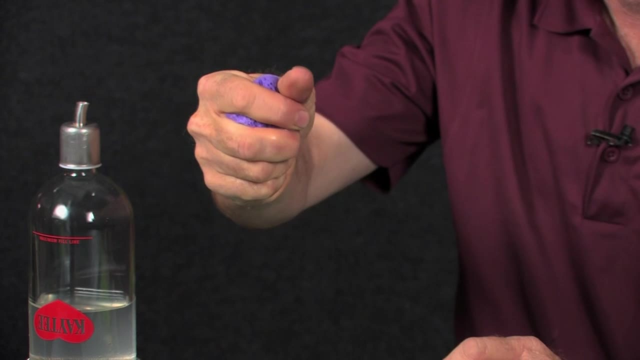 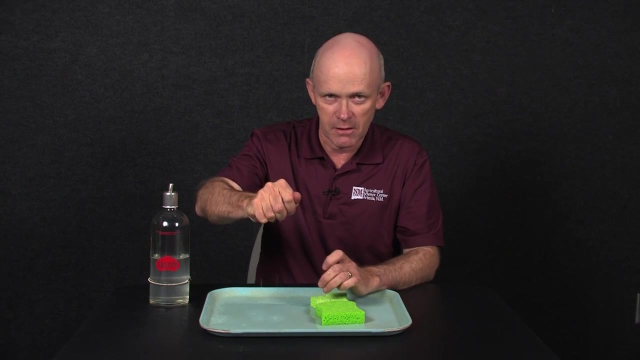 that can exert a little bit more force to actually get more water out of the soil. These are a little bit more of your drought tolerant type plants. There are other plants that can actually exert more force in order to get as much water as possible out of there, But even they. 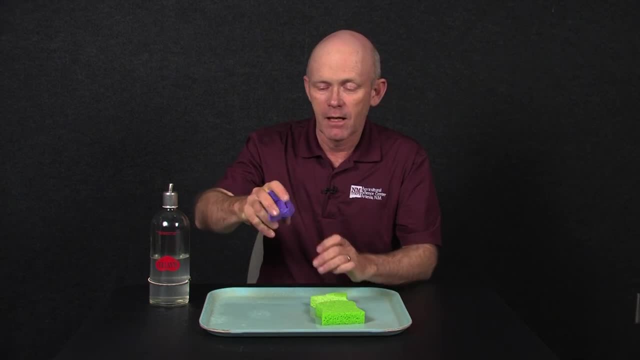 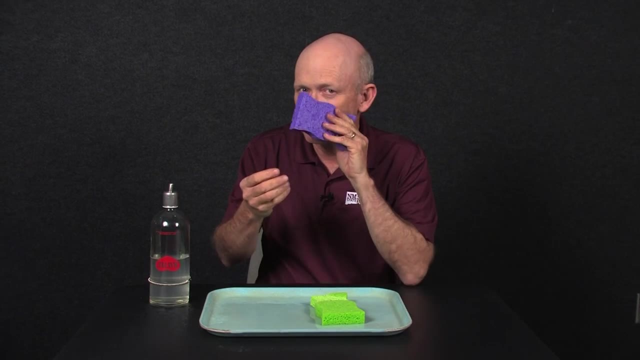 will reach that permanent wilting point. Is the sponge totally dry? Is our soil totally dry? No, It's still moist. You can feel that moisture on the soil And then it becomes even firmer. Take another look on there. but that water that's left in the soil now is so tightly held to the 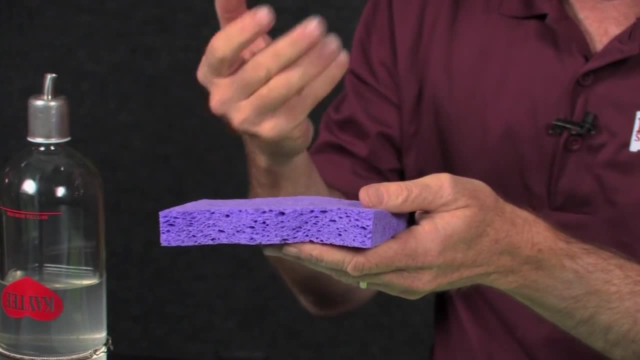 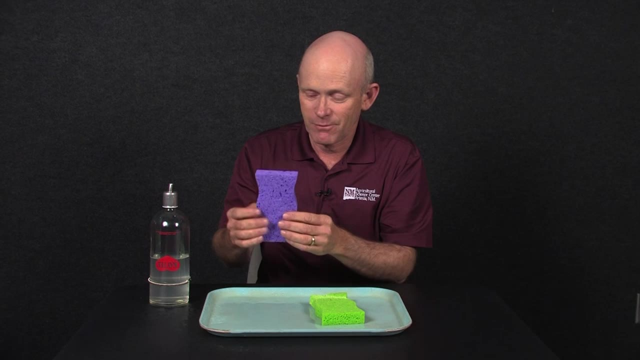 solids within the soil that the plants cannot take it out and use it. This then becomes permanent wilting point. Permanent meaning that a failure to replenish that moisture and that plant will certainly wilt and most likely die. They've used up what's known as the plant available water. This plant 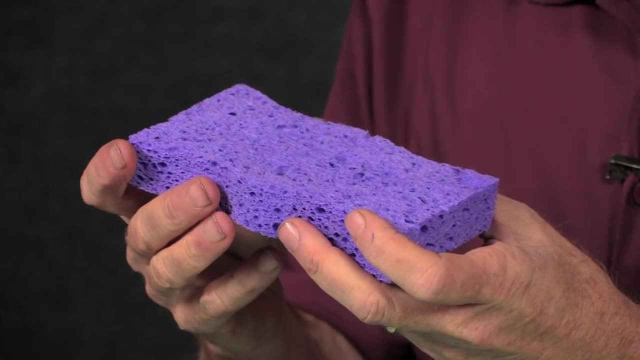 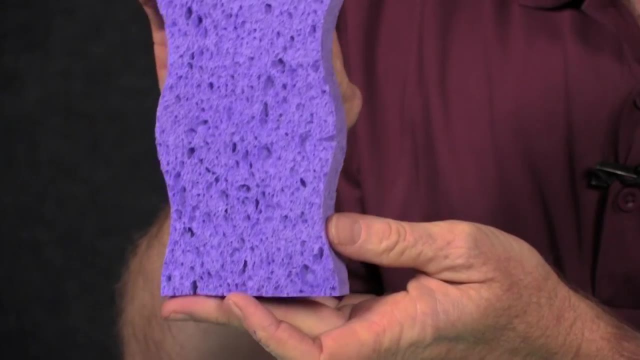 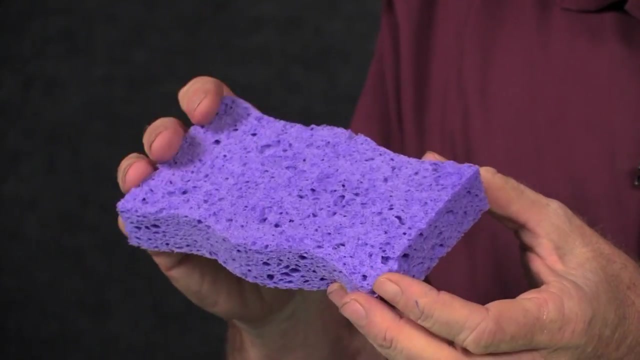 available water varies by soil texture, and the way we calculate the amount of plant available water is to look at how much water we held at field capacity and we subtract out the water that's held at permanent wilting point. Clays are actually much more similar to sands in the amount of plant available water and 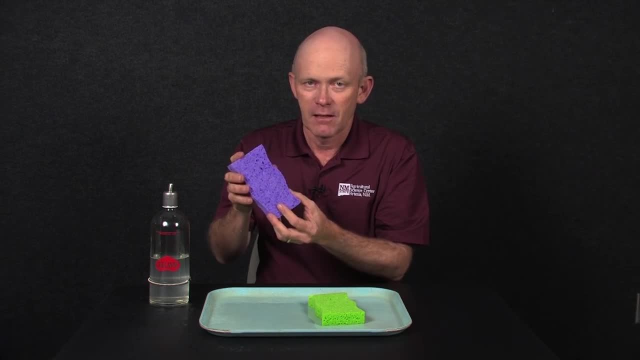 oftentimes we actually manage our water on our sands the same way as we water our soil- Clay soils- because there's still a lot of water in a clay soil but the amount of plant available water is so tightly it's just not there That plant available water. 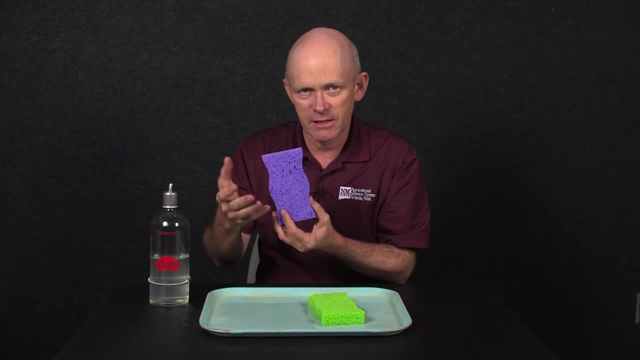 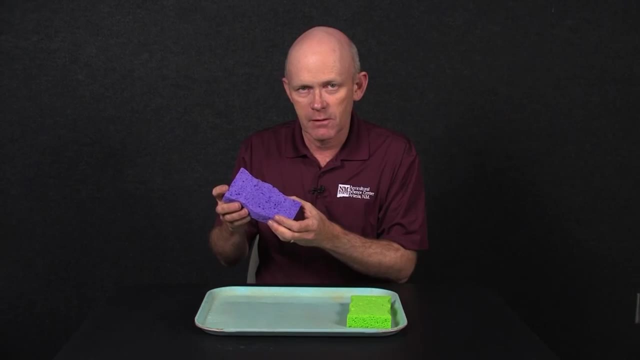 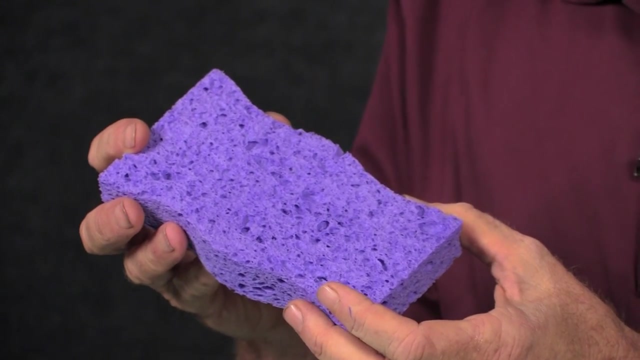 is tied up in all that solid that we see in the clay soils. The loams and the silt loams have the most amount of plant available water, That difference between field capacity and permanent wilting point, And they tend to last longer between irrigations. A lot of soils are on slopes. 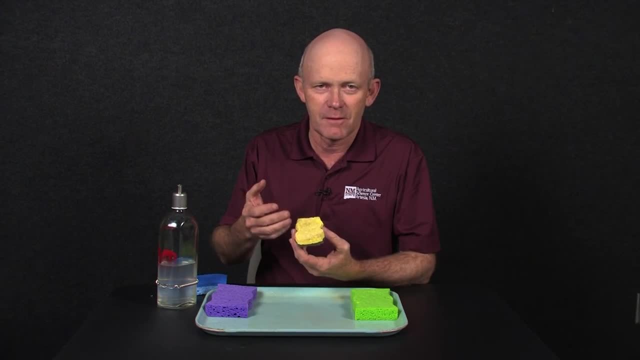 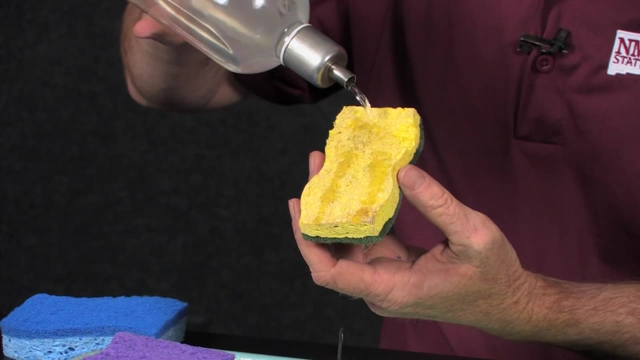 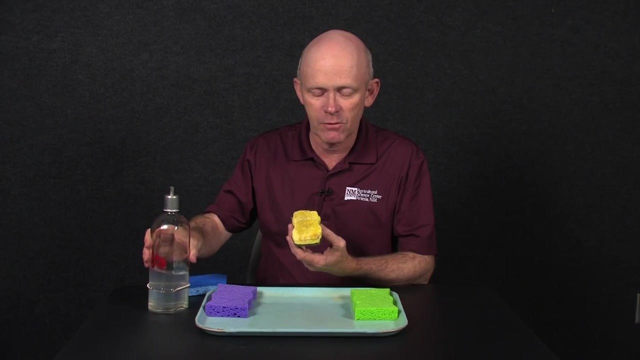 and without cover, a lot of our soils will dry out a lot, and when you first add water it may just run right off. See, just runs right off until that very dry soil starts to be wetted up. overcome that hydrophobicness These soils can get. 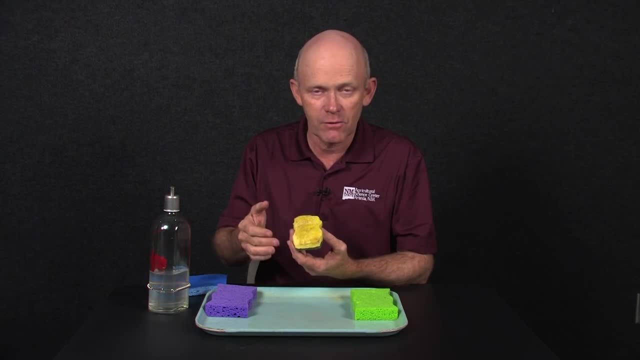 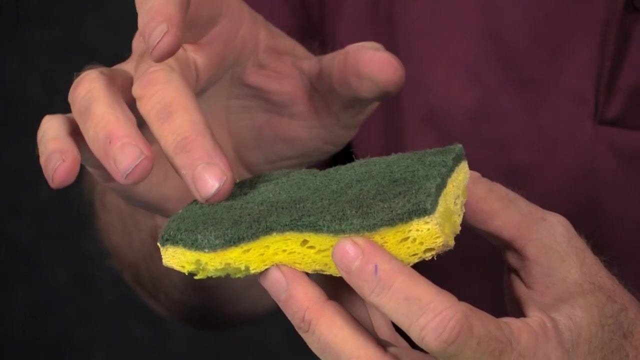 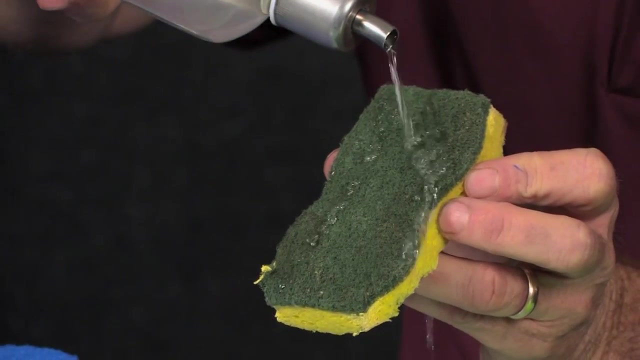 so dry sometimes that they'll actually become a hydrophobic soil. They can need time in order to start to be able to absorb water. Now, some of our soils- we could actually also have a cover on it- and our organic matter that we put on the soils can also get quite dry, and they can also run off until they 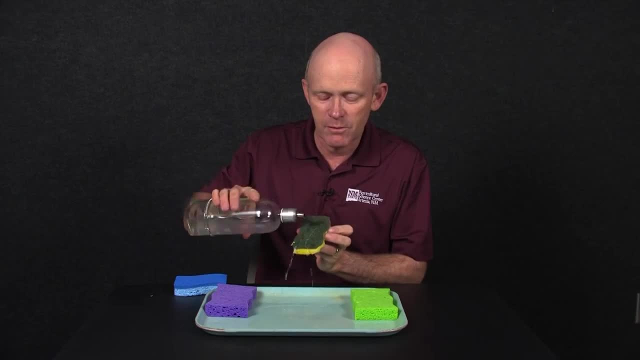 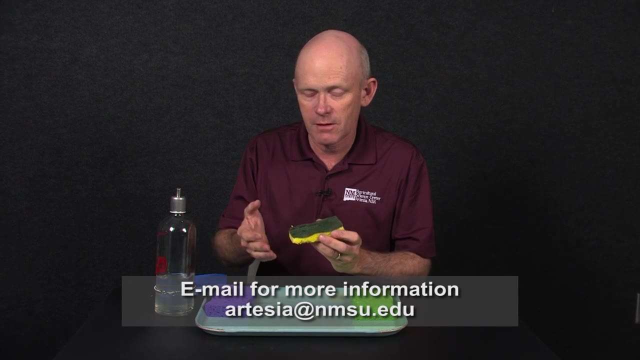 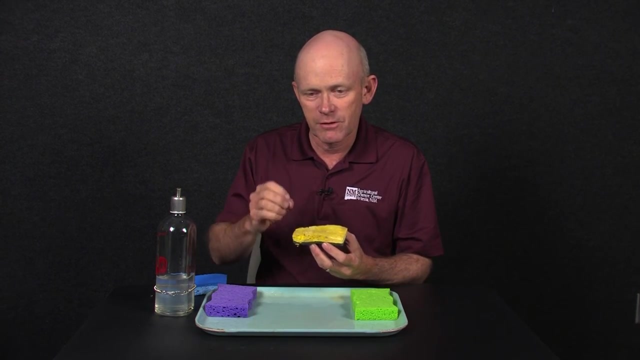 get moistened up. So we have to be wary of runoff potential for these soils and take steps of soil conservation in order to slow this water down so that it can start to go into the soil and not run off and bring soil particles with it. So these 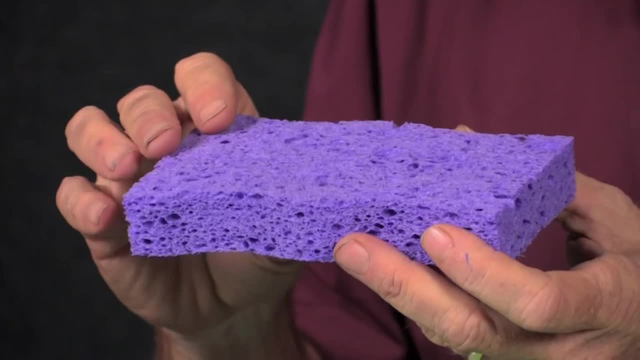 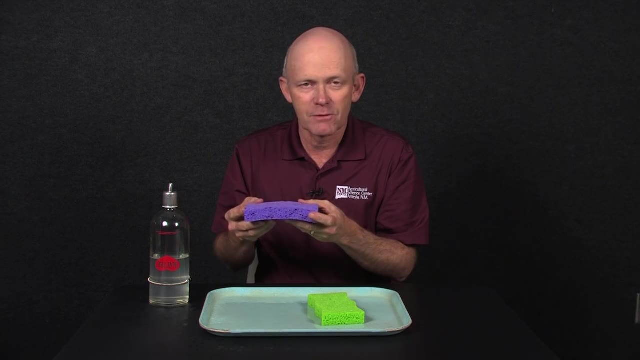 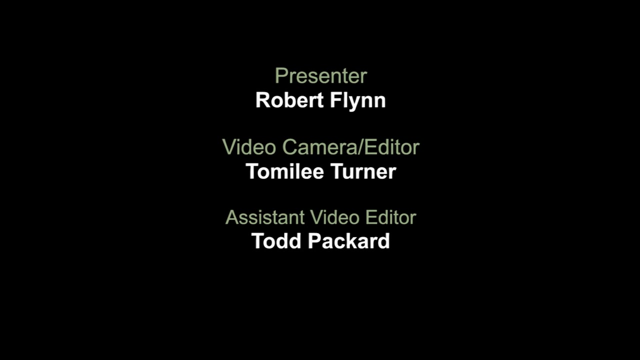 are the key properties of soil texture as it relates to water movement and pore spaces, and how they affect the water holding capacities of soils. you